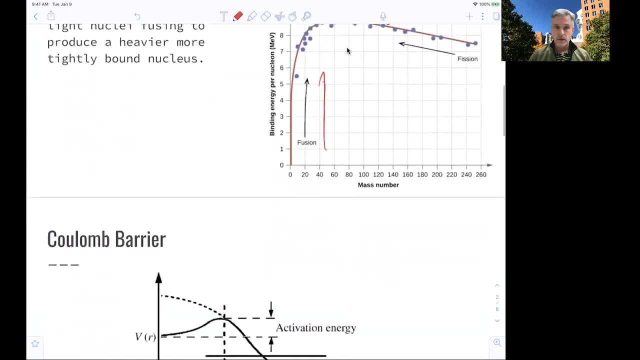 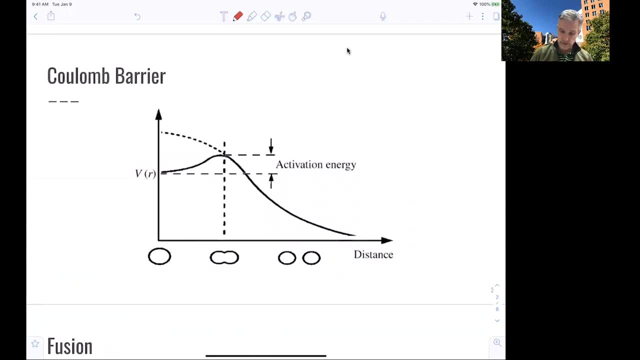 empirical mass formula. OK, so the difficulty in nuclear fusion is that we now have to overcome the Coulomb barrier from the other side. So we have to bring two light nuclei together, have to overcome the Coulomb barrier in order to form this heavier and more tightly bound. 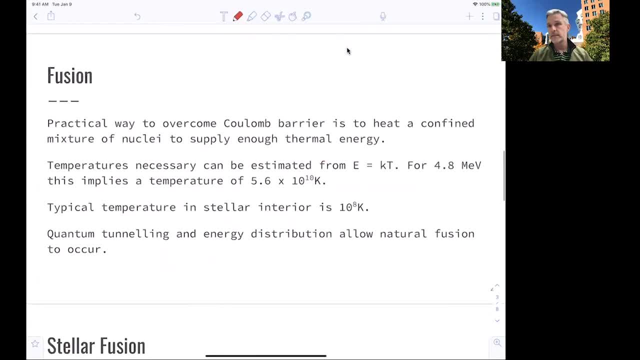 state. You might think that you can just take two beams of protons, like we do at the LHC, bombard them and create heavier nuclei. But the problem is that most of the nuclei will scatter elastically and will not lead to a new bound state. So the practical way 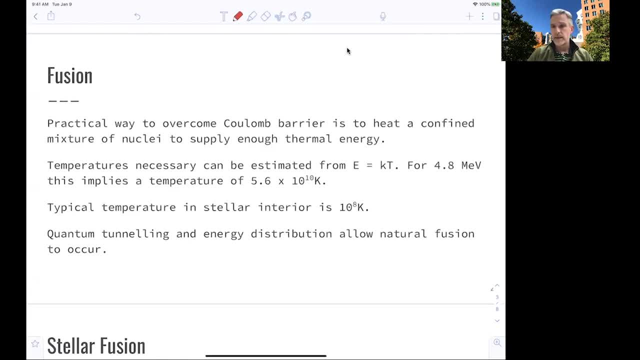 to overcome the Coulomb barrier is by creating a confined mixture and supplying heat such that the thermal energy is enough to overcome the Coulomb barrier. Now you can estimate how much energy is needed If you, for example, assume a Coulomb barrier. 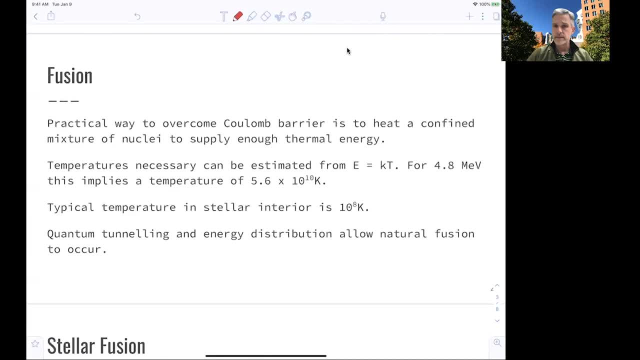 of about 5 MeV. this implies temperatures of 5 times 10 to the 10 Kelvin. OK, so that's really really hot, right? If you compare this to typical temperatures within stars, you will find that those are only 10 to the 8 Kelvin. 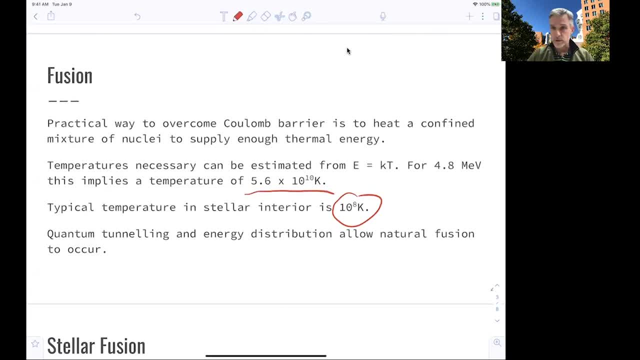 So now you ask: what is the temperature of the Coulomb barrier? Why does it still work? Why do we see fusion within a stellar medium? And the answer to this is again quantum tunneling and to some degrees also the fact. 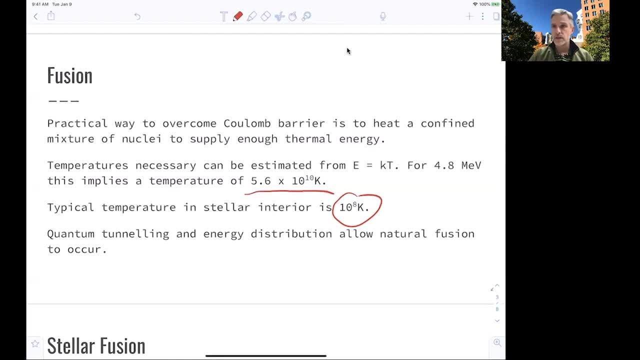 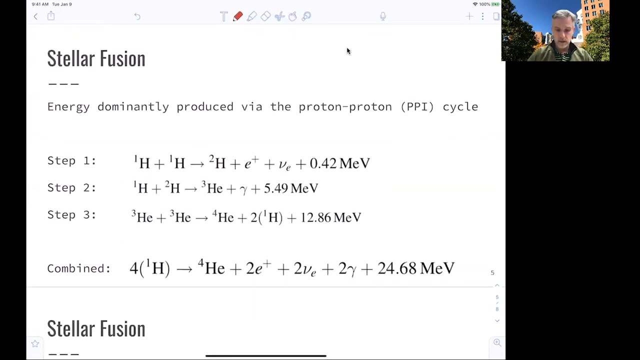 that when we have a medium of a specific temperature, the kinetic energy of the particle involved follows a maximum energy distribution. So you find some particles which have enough energy to overcome the Coulomb potential. Even so, the mean value would be below The processes within the sun. they are dominated by so-called proton-proton cycle or PPI cycle. 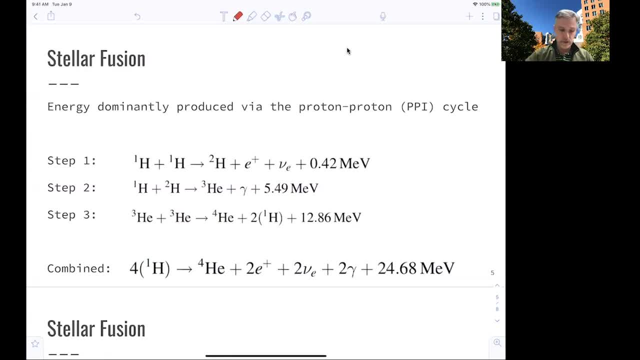 And this happens then in a number of steps. You start with hydrogen or protons. You know, the core of the sun is basically a plasma, So we can forget about electrons in this context. So we have two protons fusing together. 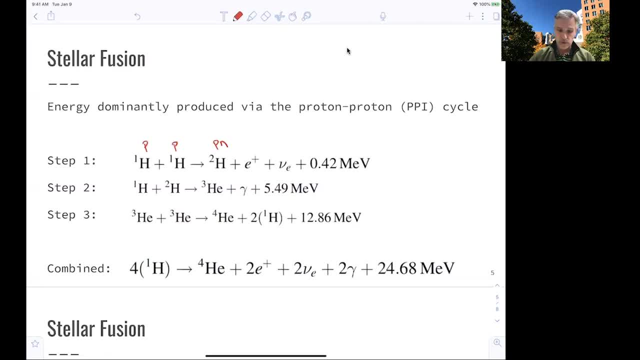 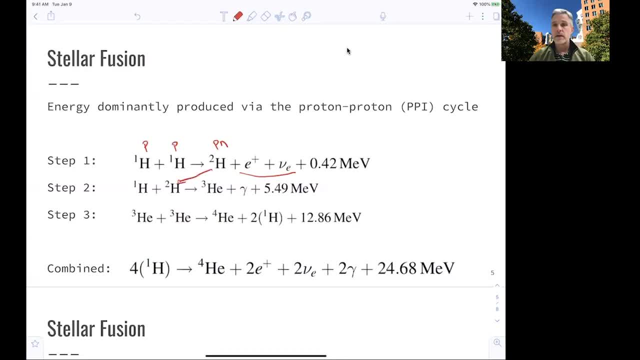 Then you supply the deuterium again And together with the proton you are able to produce the helium, And then the helium again is being used to supply the third step in this: Helium-3 is supplied to produce helium-4.. 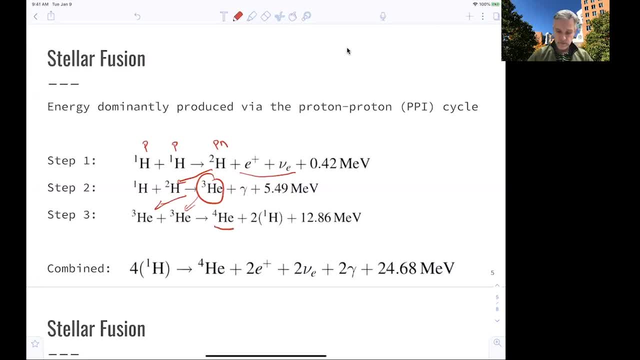 So this is then. the end product is the helium-4 here and energy. If you combine all of those three steps, you find that you start with four protons. You produce helium-4, positrons, neutrinos, photons and energy. 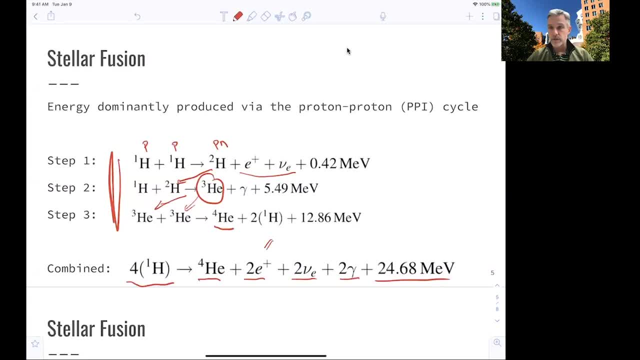 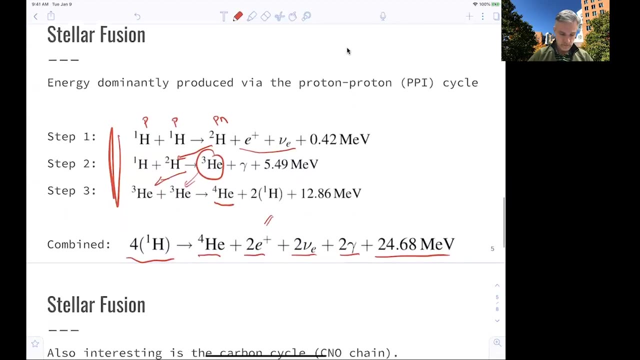 In fact, as I was just saying, this all happens within a hot plasma. The positrons are basically annihilated with electrons, which are part of the plasma, adding another MeV of energy to this. All right, this is one and the dominant energy production. 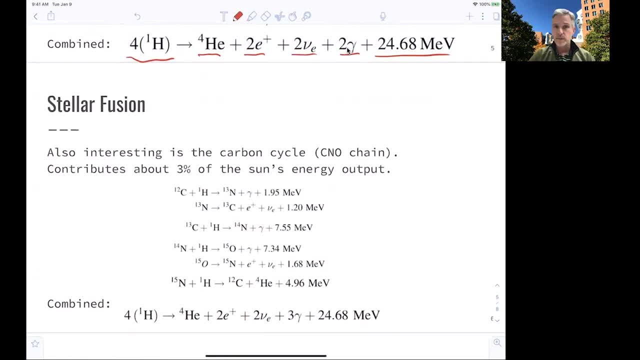 mechanism within the sun, but it's not the only one. Also quite interesting is the so-called carbon cycle. It's contributing about 3% to the sun's energy output, So here carbon basically works as a catalyst. So you have a carbon. 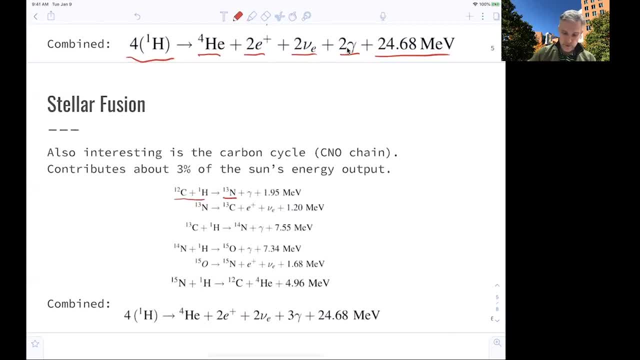 And again a proton producing nitrogen. The nitrogen produces carbon-13.. Carbon-13 together with a proton, Nitrogen-14, nitrogen-14 with a proton, Oxygen-15, and oxygen-15, nitrogen-15.. And then, last but not least, nitrogen-15 together. 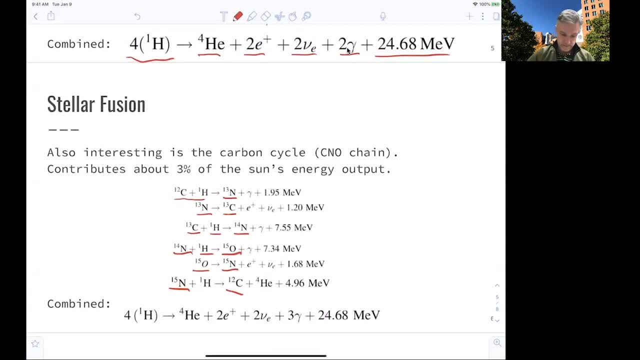 with a proton, produces carbon-12 again and helium. So you see that the carbon-12.. Carbon-12 is the catalyst here which is used to produce helium and energy. So if you produce this cycle, if you combine this cycle, 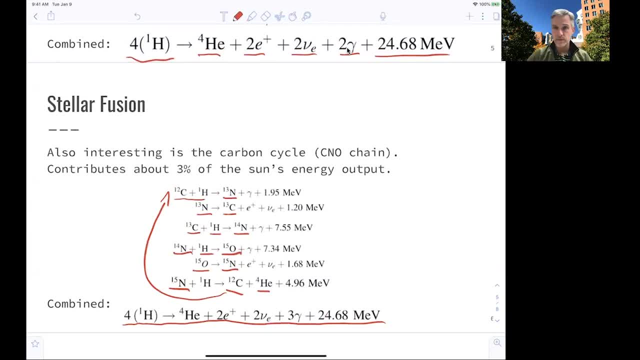 you find that again from four protons or four hydrogen atoms you produce helium positrons, again neutrinos, three photons and energy Very similar. It's still visible to this combined chain, with the exception that there is one additional photon. 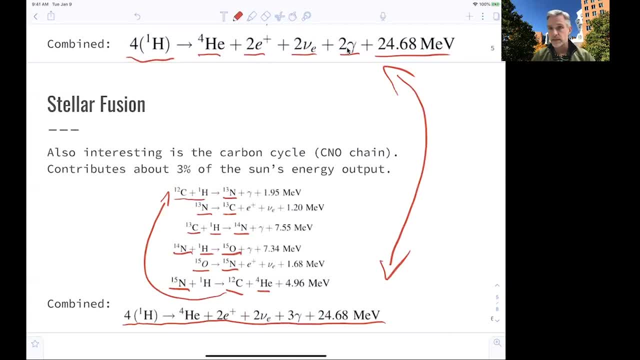 And again, here And here, the positrons supply additional energy And they annihilate with electrons. Great. So we have seen that we do two things: We create heavier forms of matter, starting from hydrogen, And we produce energy, And so this is the energy production. 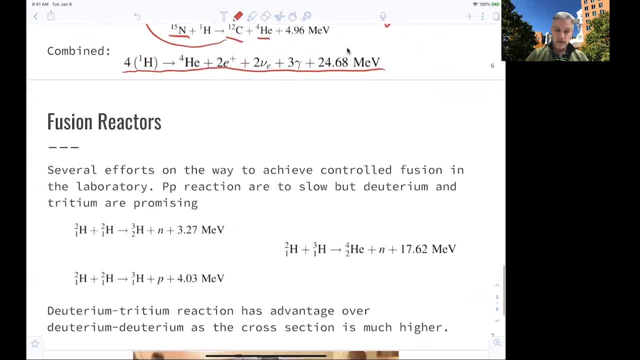 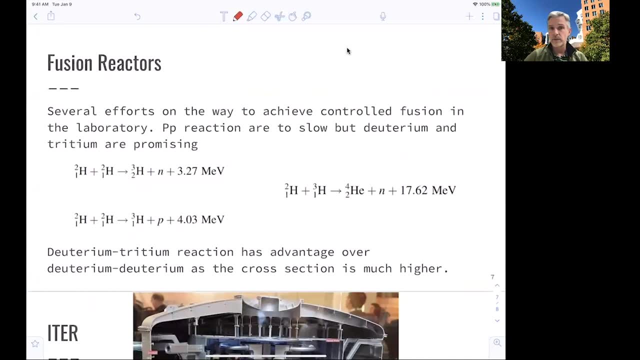 mechanism within the sun. This is nice, You know, you produce. You start with hydrogen or deuterium- Those are two elements which are very abundant- and you produce energy. So the question comes up whether or not you can actually use this on Earth. 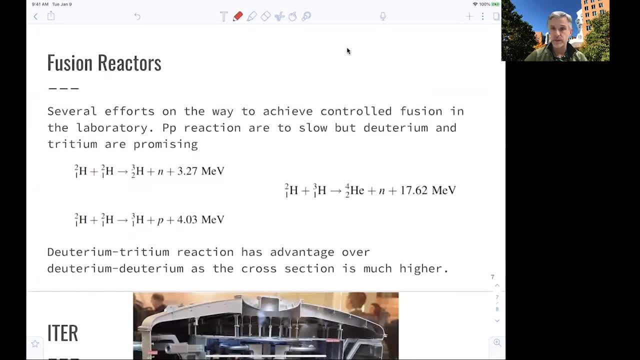 in a controlled environment in order to produce energy and solve many of the ongoing issues we have on this planet. There are several efforts on the way, And this goes back all the way to the 50s of the last century. The most prominent one currently is the so-called ITER project. 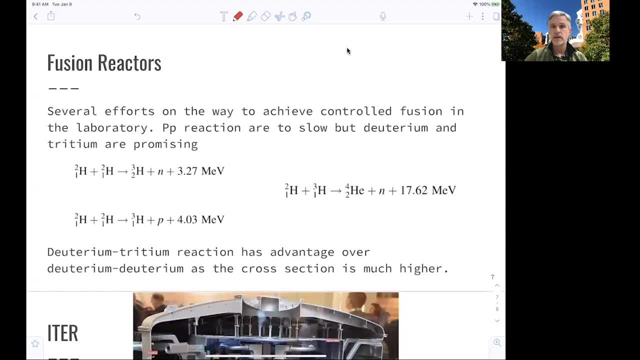 which is an international collaboration and a project where one tries to build a fusion reactor in France. I can only tell you that the next stage for this is in about five years to complete the project, or complete the construction of the project and produce energy for the first time. 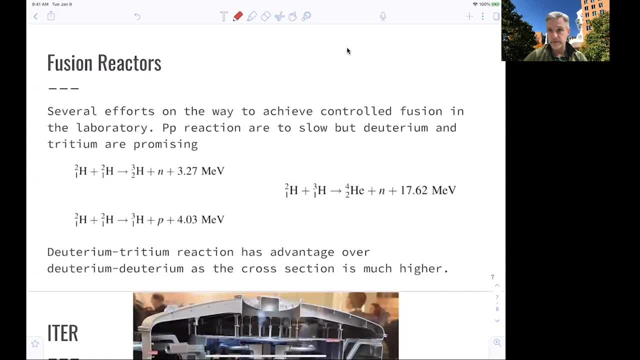 with this project in this controlled environment. It will take another 10, 15 years on this roadmap of research in order to produce It will be able to produce nuclear power reactors, nuclear fusion power reactors, which can be used in some sort of commercial way. 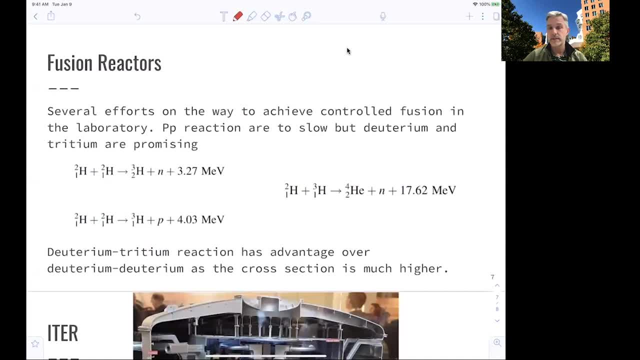 There's a few other interesting projects which use different magnetic technologies which might have a more faster pathway to success. Coming back to the story here, so you could start with protons again in a proton-proton reaction, But it turns out that this is a rather slow process.